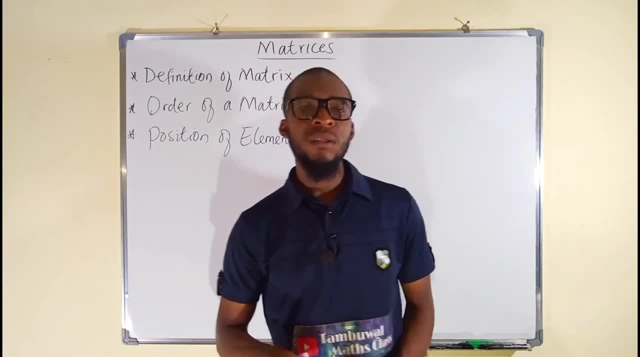 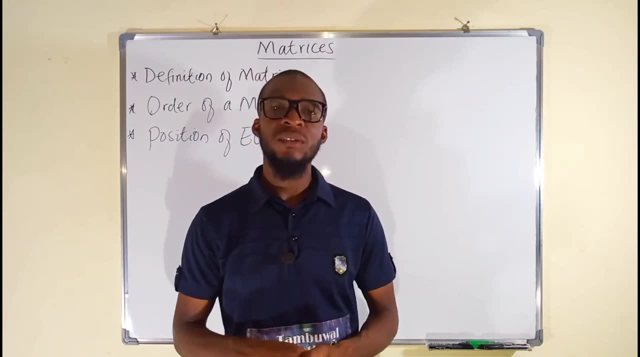 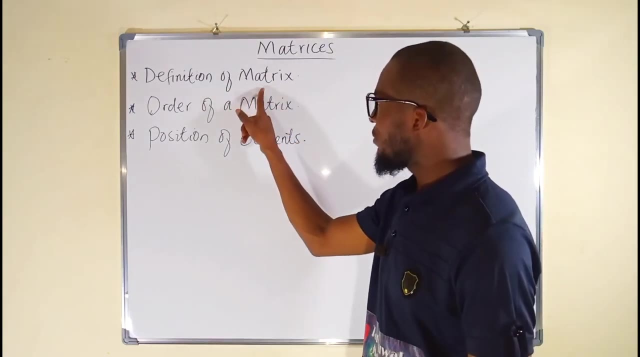 matrix. So if you are new here, consider subscribing. press the bell icon so that you will be notified whenever I upload a new content, and don't forget to share to your learning colleagues. Now let us begin with the first one: Definition of a matrix. This matrix is just the singular form. 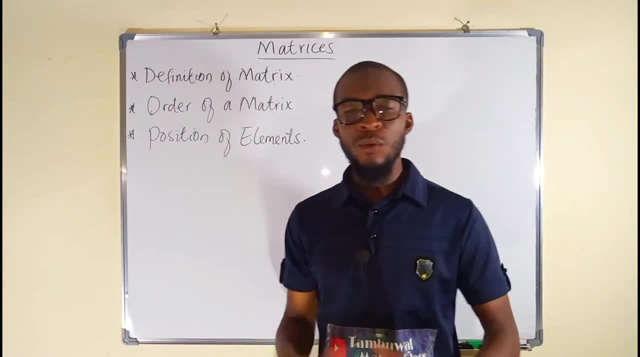 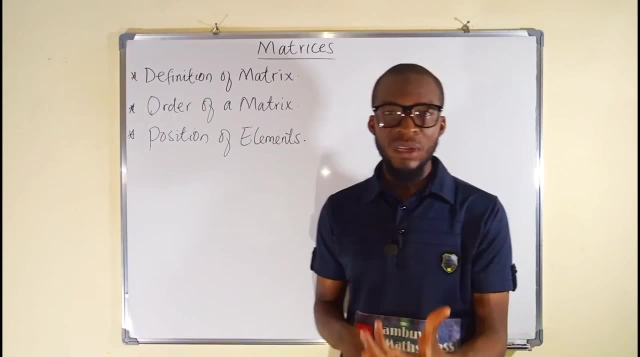 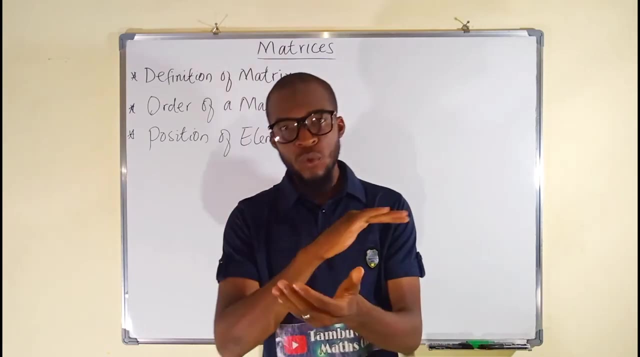 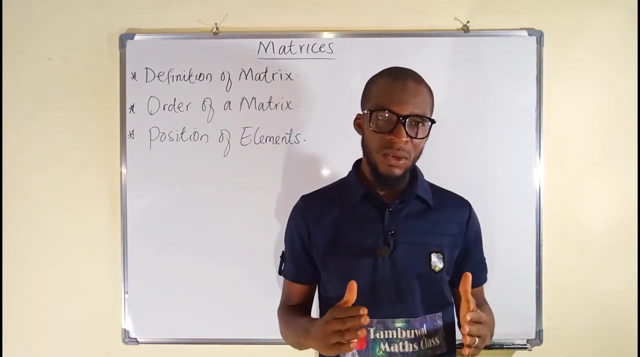 of matrices. Matrices is the plural form. A matrix is a rectangular arrangement of elements, and these elements could be numbers or even characters, Arranged in a particular number of rows and columns. This matrix is a matrix of numbers and even characters. A matrix is represented by an uppercase letter, while the elements in a matrix are donated by. 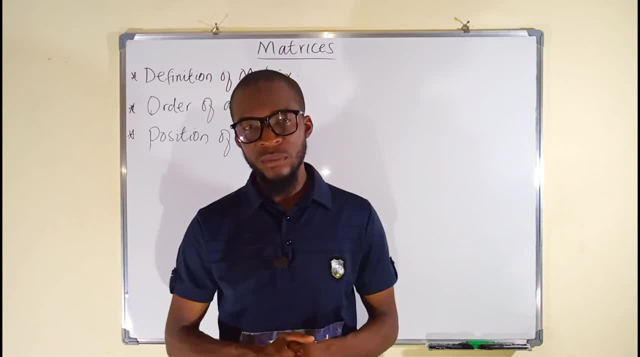 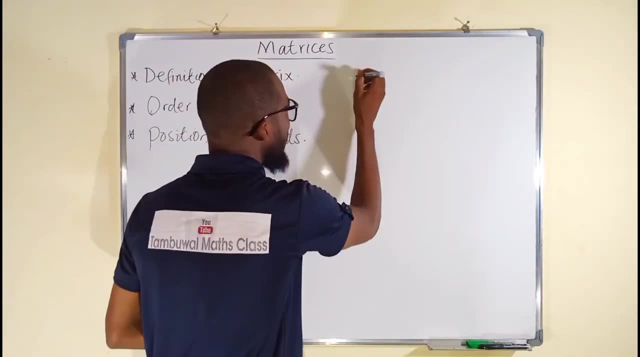 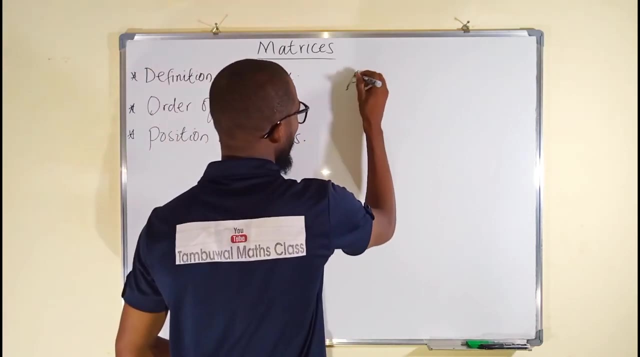 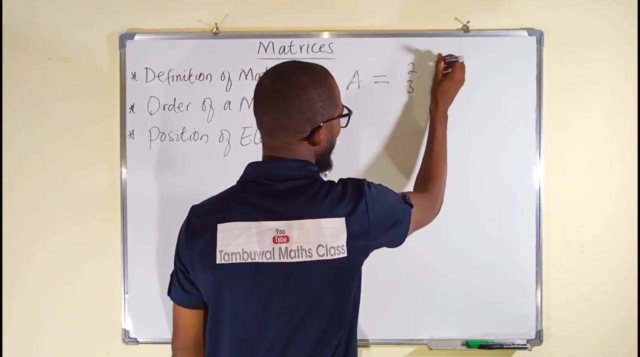 lowercase letters if dealing with variables. So now let us see how we can represent a matrix. Suppose we have a matrix A- Remember it is donated by a capital letter, sometimes written in bold form. Suppose this is a matrix of numbers. Choose the digit letters used in the matrix and focus on that basic matrix. 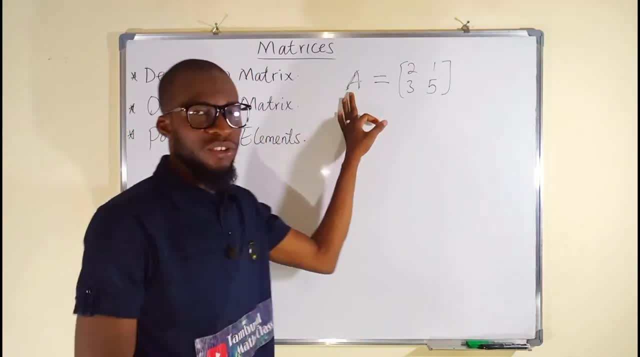 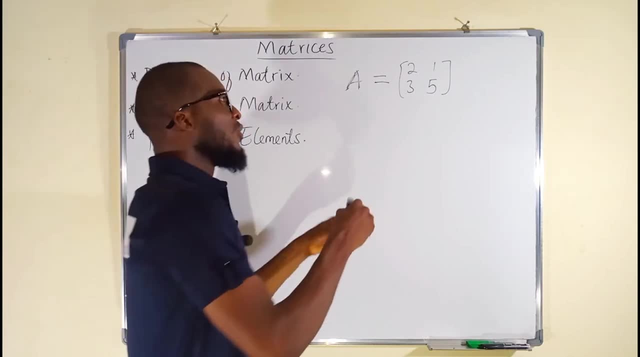 Picture of A matrix. Take a look at the bases of A matrix. for example, 2, 3, 1, 5.. 2,, 3, 1 and 5 are said to be the elements of this matrix A. 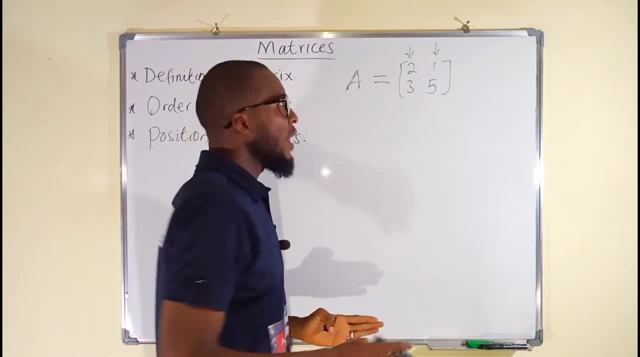 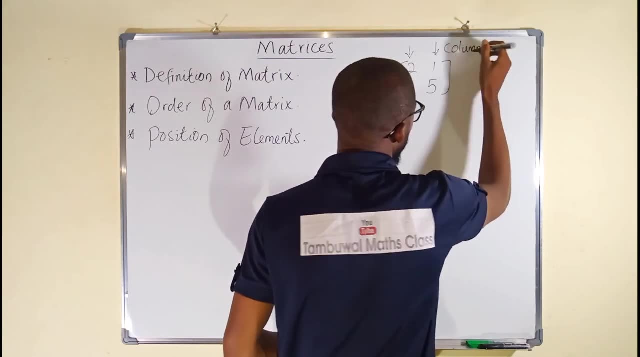 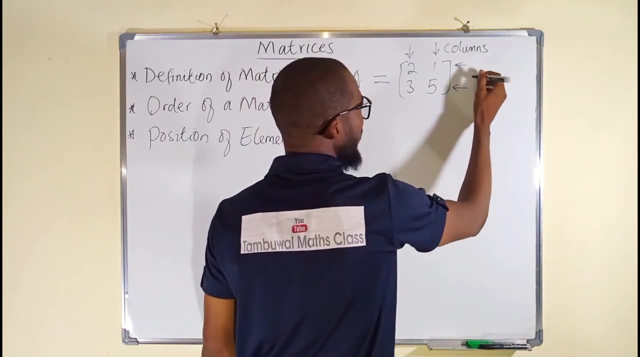 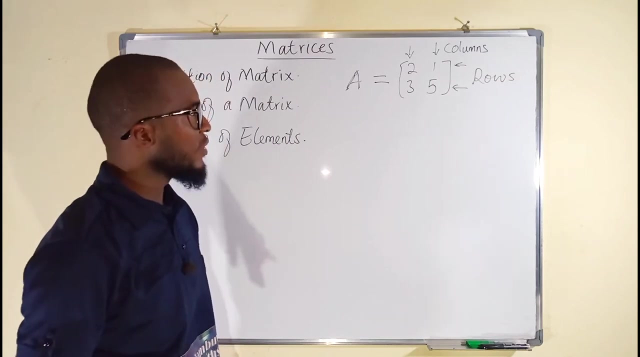 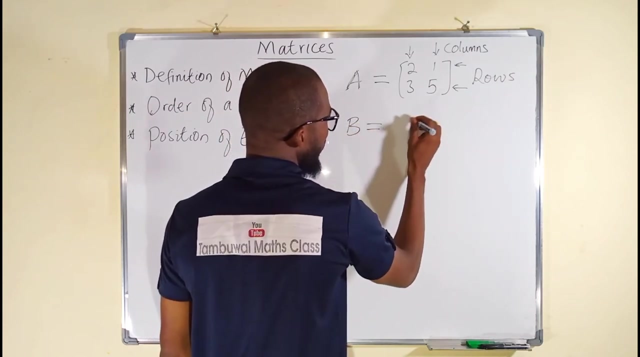 And they are enclosed under a bracket, So are said to be the columns. so we have columns. we have two columns, while these ones horizontally are said to be the rows. so we have two rows and two columns in this particular matrix. we may have another matrix, say b of the latest, a, b and c. 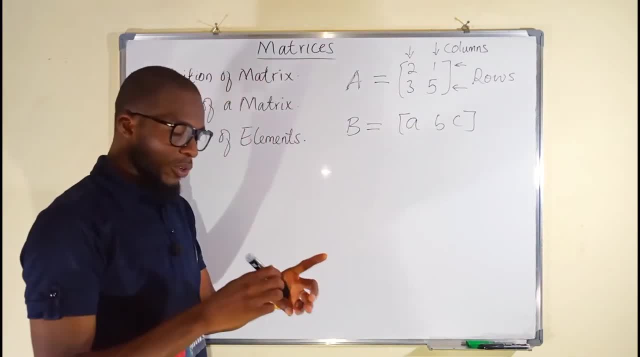 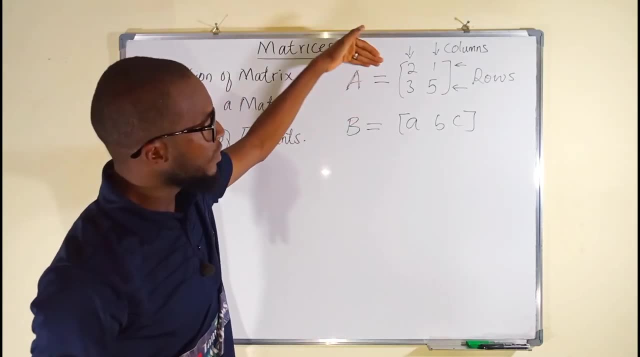 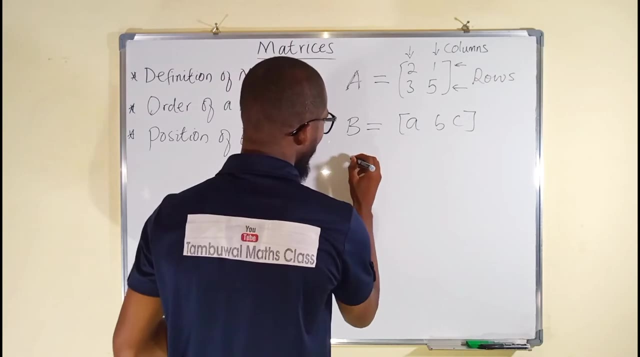 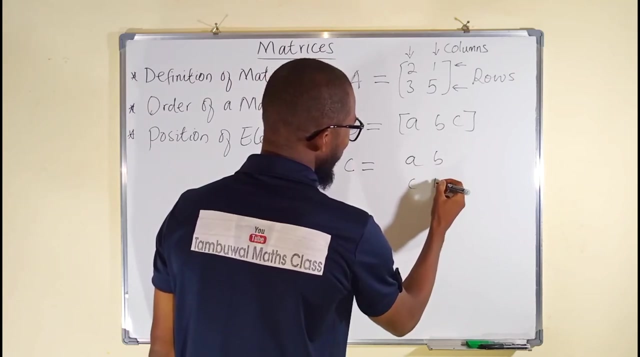 in this form, so a matrix must not be necessary. all in the same format. you can see, this one has two rows, but this one has only single row, but three columns. we may have another matrix, c of the form, maybe a, b, c, d, e and f. this is a matrix. 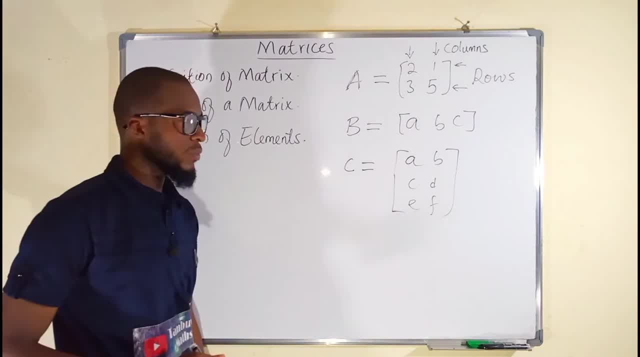 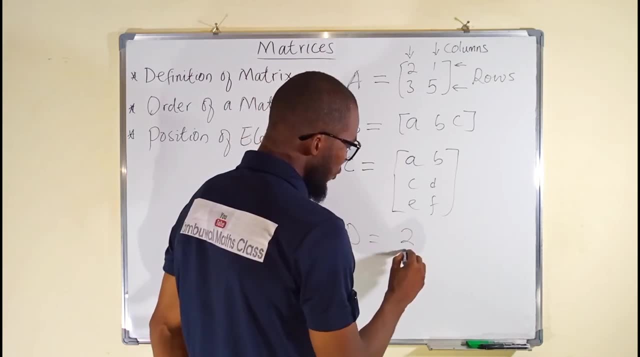 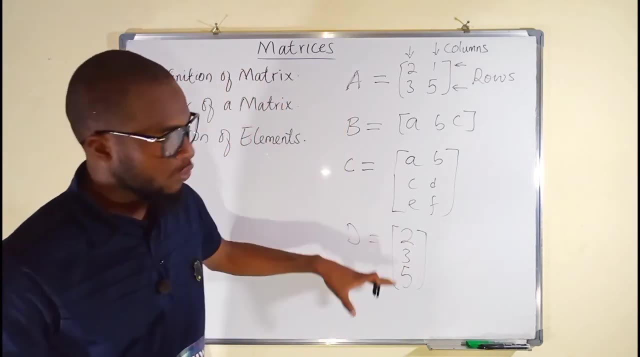 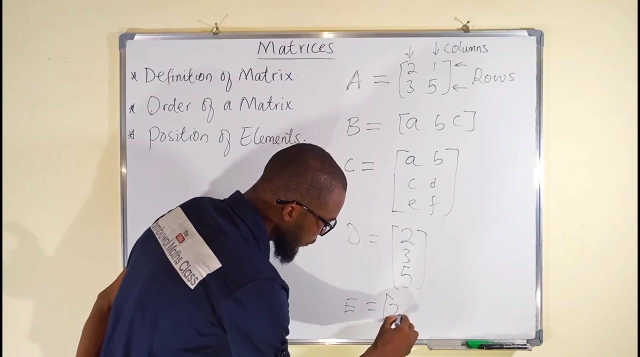 of three rows and two columns. we may have another matrix like this of numbers like, say, two, three, five, only having a single column, where you can see we have three rows. you may even have a single element in a matrix. this is also a matrix. so this is how a 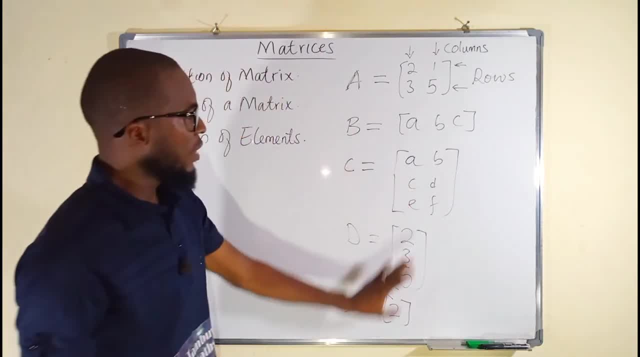 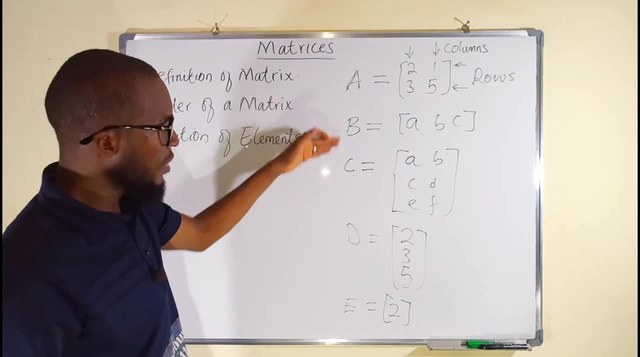 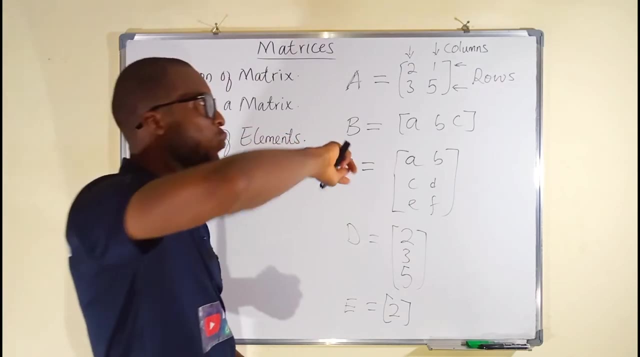 matrix is represented under a bracket and those elements under the bracket are said to be the element of these matrices you have. we have a, b, c, d and e, and vertical arrangement are said to be the columns, while the horizontal arrangement is said to be the rows. so this is all about. 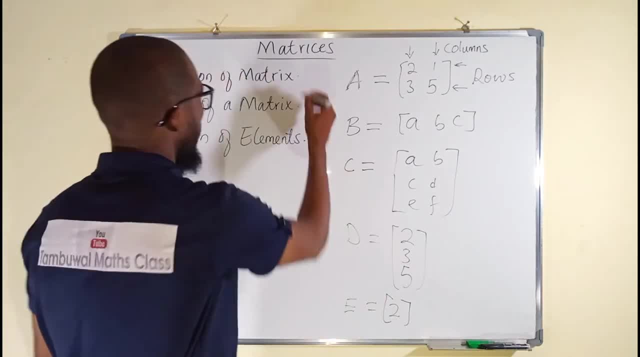 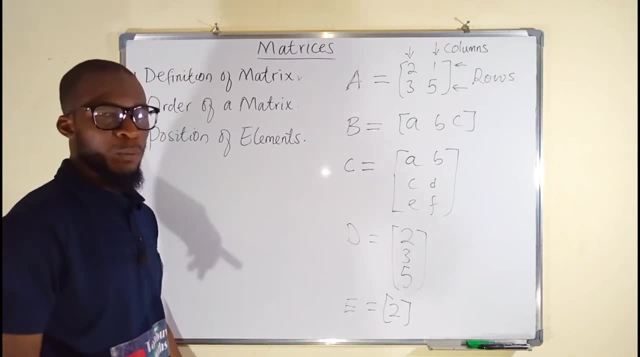 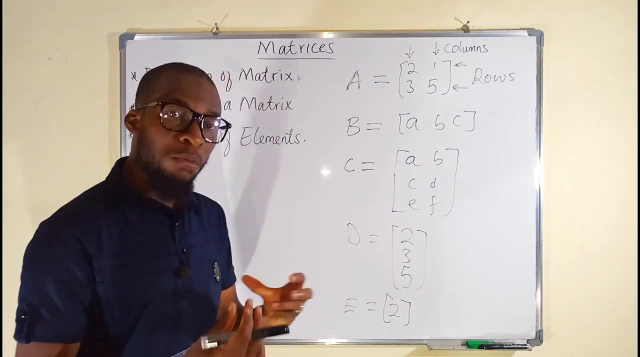 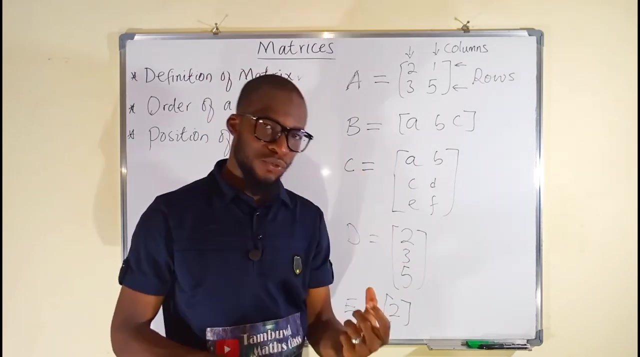 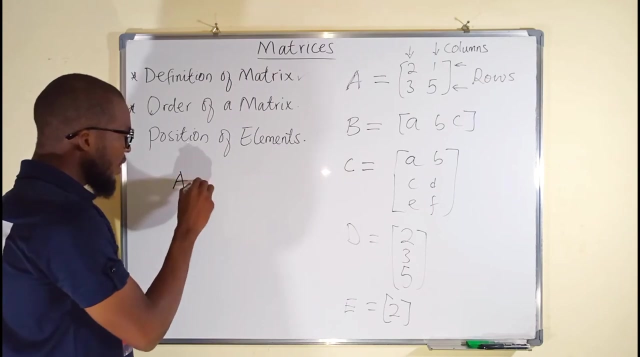 definition and representation of matrix. let us talk about the second one, which is the order of a matrix. the order of a matrix is just the dimension of that particular matrix according to the number of rows and columns in that particular matrix. always, you have to start from the rows, followed by the columns. now let us talk about a, a matrix. a is of the order two by two. 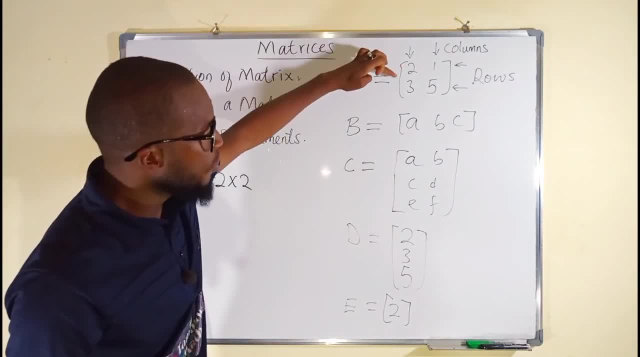 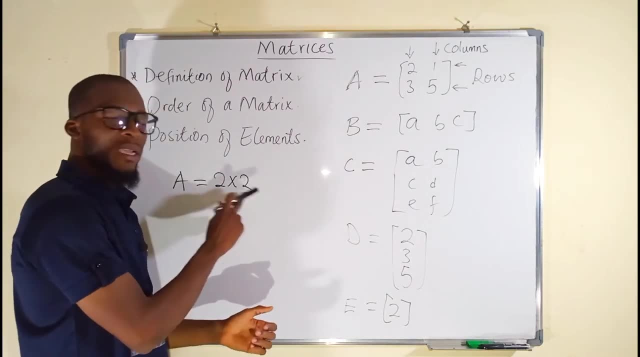 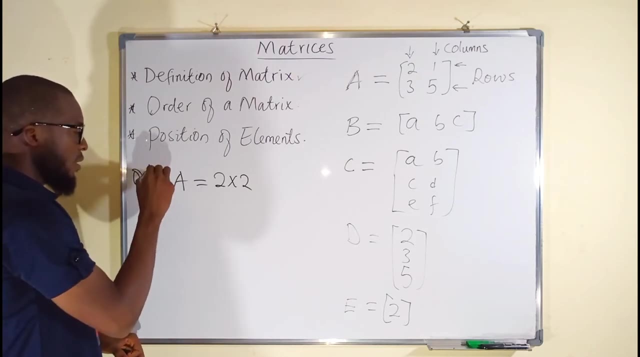 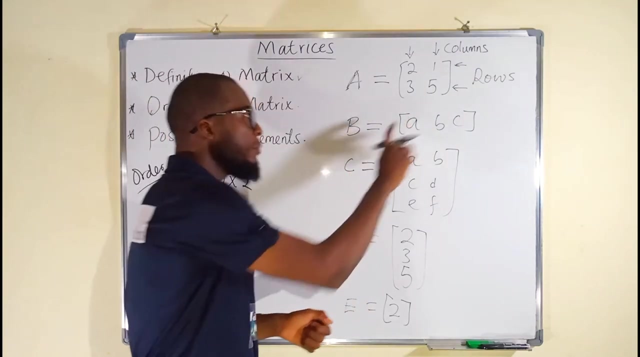 why? because this matrix has one row, two rows, one column, two columns. so the number of rows by the number of columns. we are talking about order. let me even write it here: order of a matrix. matrix b is of the order one by three. this is one by 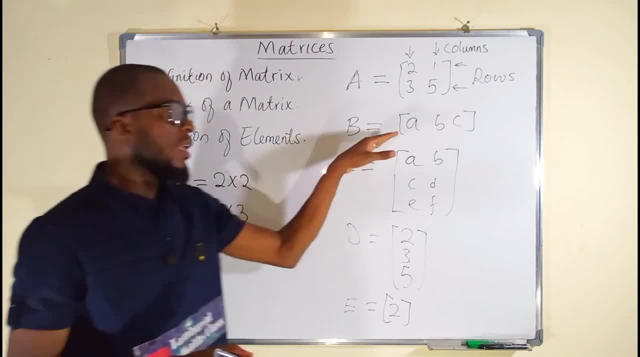 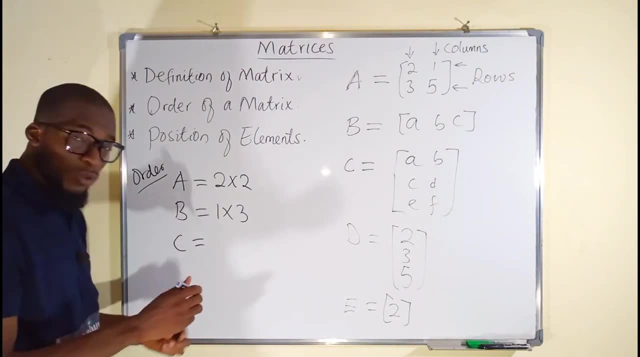 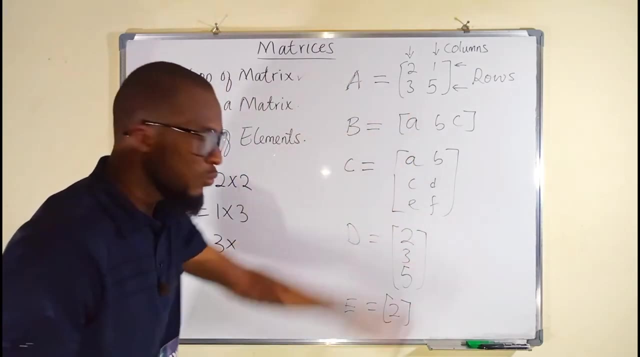 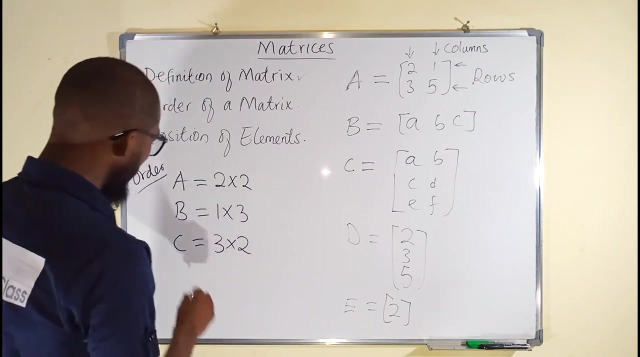 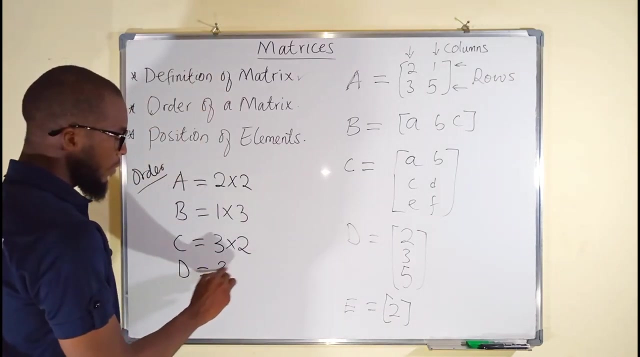 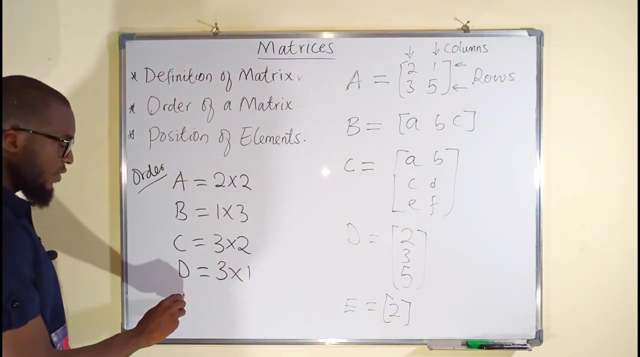 three because it only has a single row but has three columns. mattress c- you're talking about oldest- one, two, three. so this is three by one, two. remember always start from the rows followed by the columns. mattress d is one, two, three by one because it only has a single column. and last but not the least, which is mattress e. 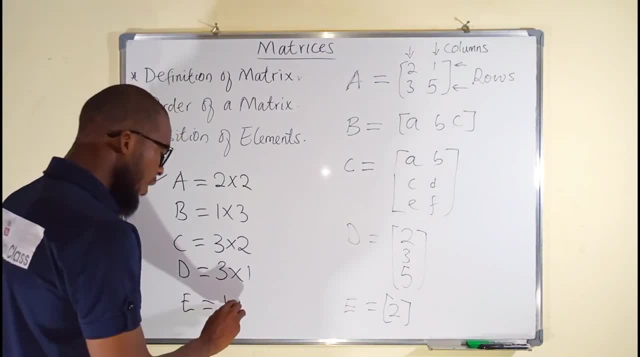 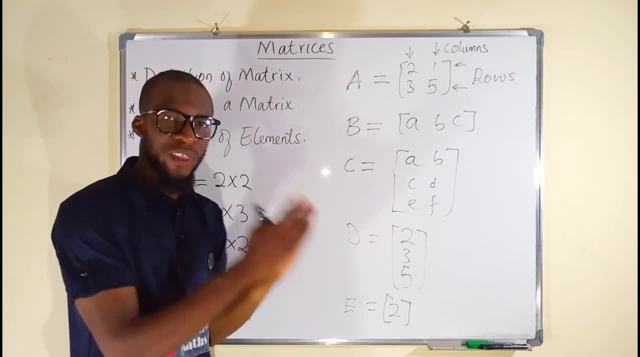 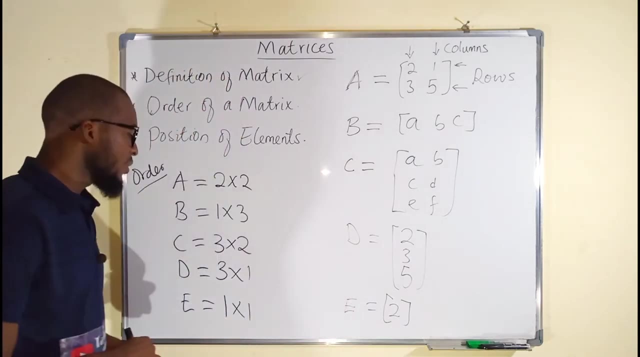 has only one row and one column. so this is all about. order of matrix is just the dimension of that particular matrix according to the number of rows, anger and all correct form and measure, Em vo organizing, which means as long sensors and and column of that matrix. position of elements. coming to the last one, 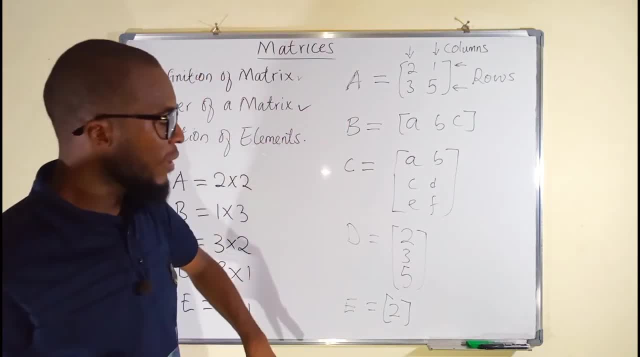 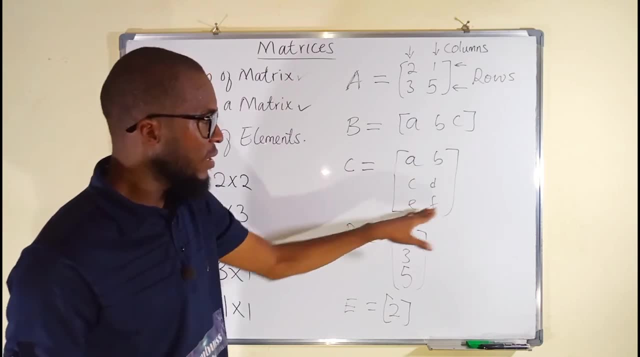 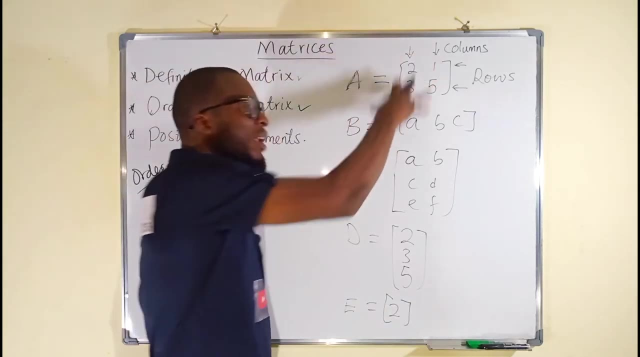 position of elements in a particular matrix. remember, i told you these are the elements. we have two, one, three, five. here we have a b c, we have a b c, d, e, f. we have two, three, five, we have two. all this are said to be the element and each element in a particular matrix is said to be. 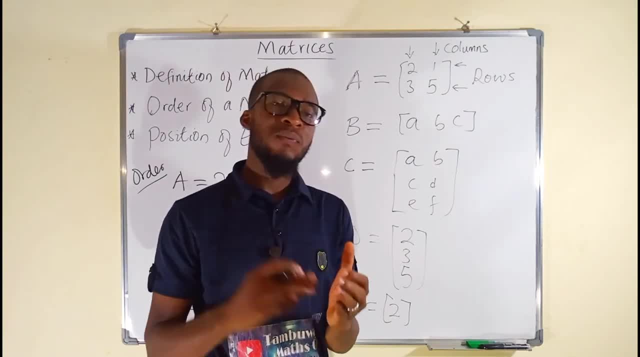 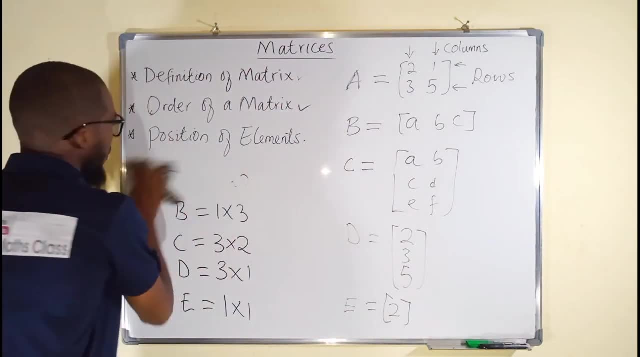 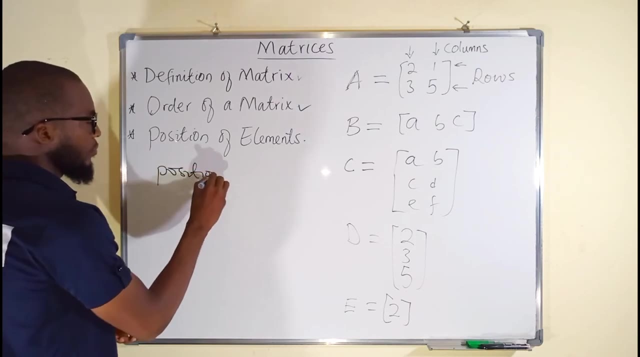 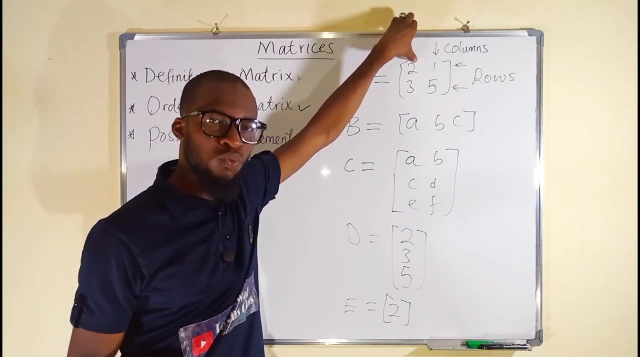 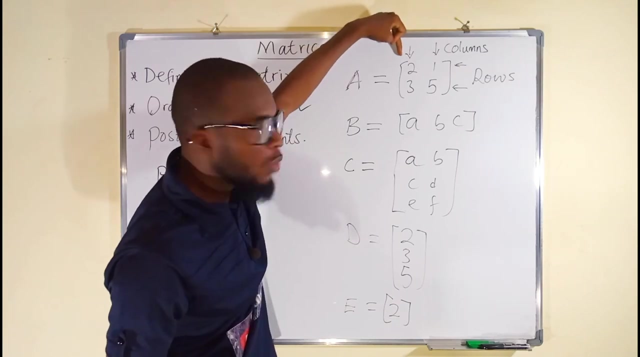 unique meaning. it has a way of identifying that particular element along. okay, coming to position, let's consider this matrix a. this matrix a has four elements, but what is the position of these two? this two, you can see, it is from the first row and first column as well. one is from the 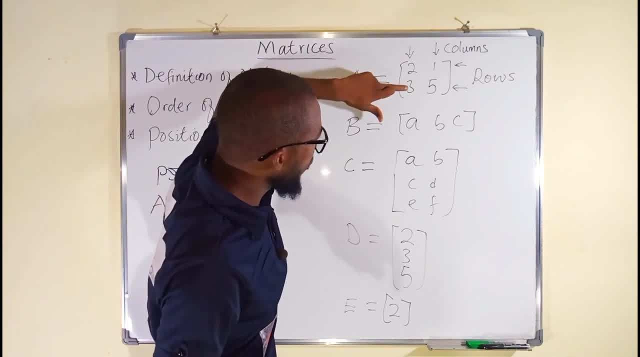 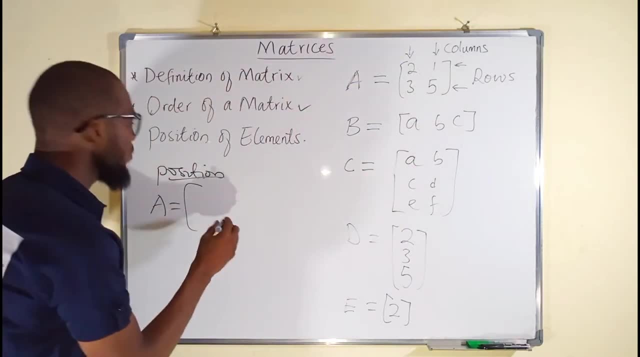 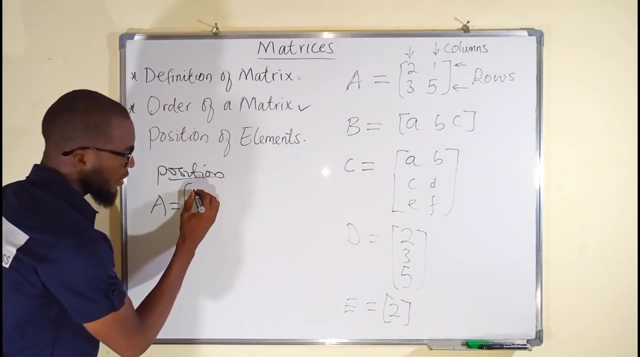 first row, second column. this is second row, first column, second row, second column. so this is how to identify each element there, so we can represent them, and this order can be written in subscript form. let me show you how. uh, the first element, the top left corner, is a 1: 1, followed by a 1: 2, followed by a 2: 1, then a 2: 2. 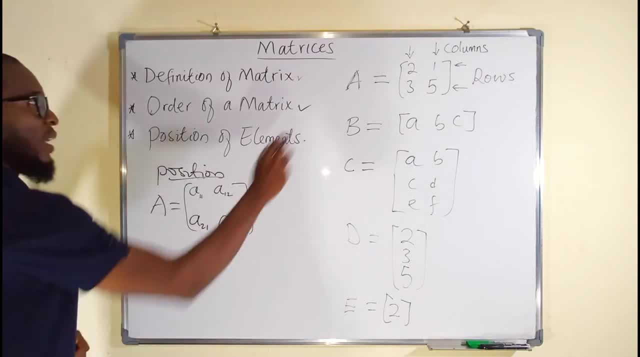 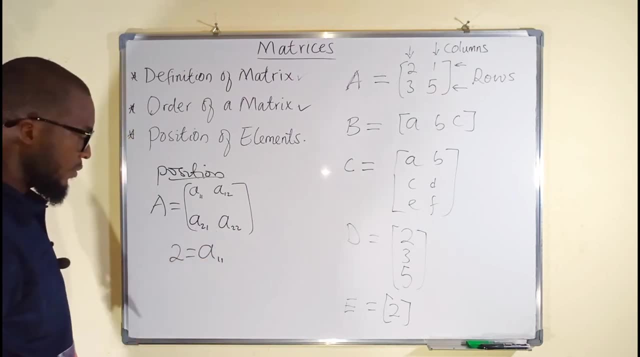 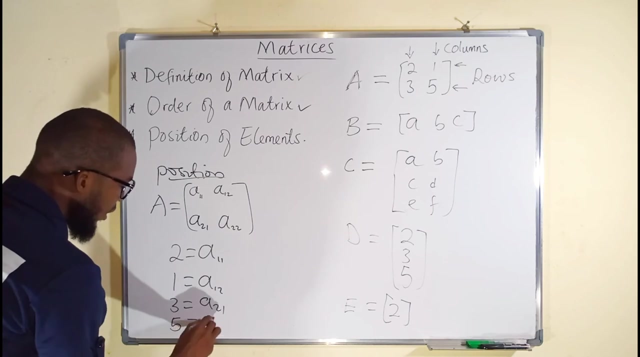 so now, if you relate this matrix to this matrix, 2 is said to be a 1, 1 that the sub-symbol is should be in one 때. 1 is said to be a one. two, three is said to be a 21 under five plus, but not the list is said to be a. 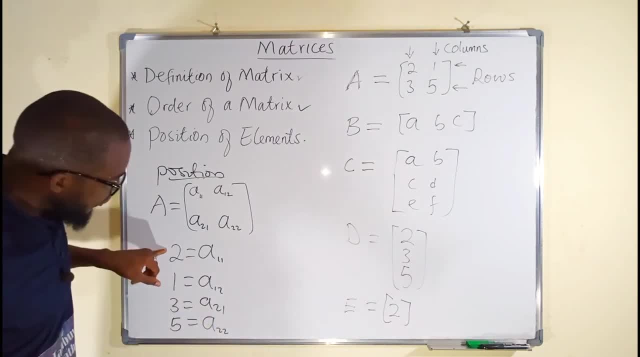 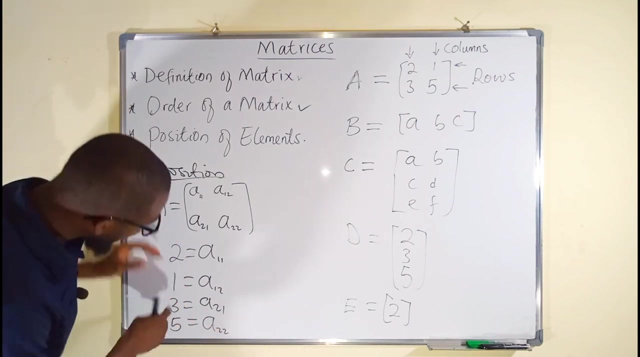 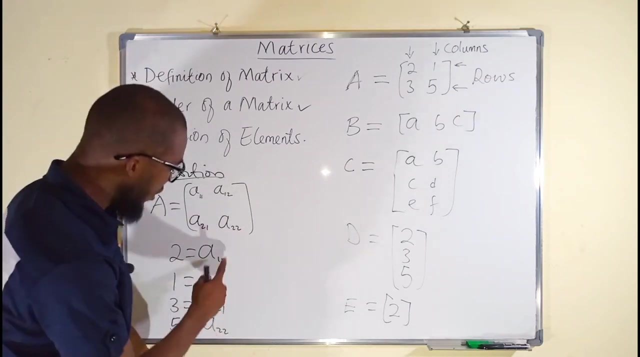 22. what does this mean? it means that two is an element at first row, first column. one is also an element at first row, second column. three, second row, first column. five, second row, second column. so you can see, they are unique, because none of this representation is similar to another. they are all unique. this is. 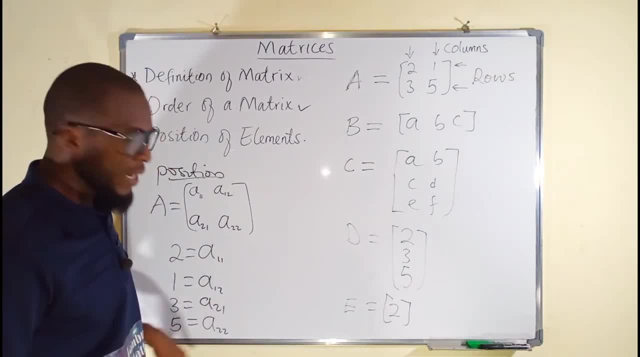 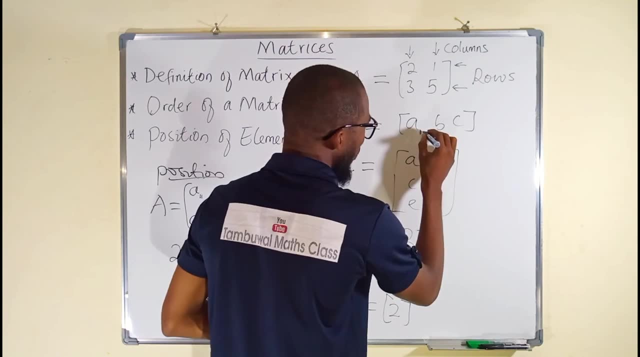 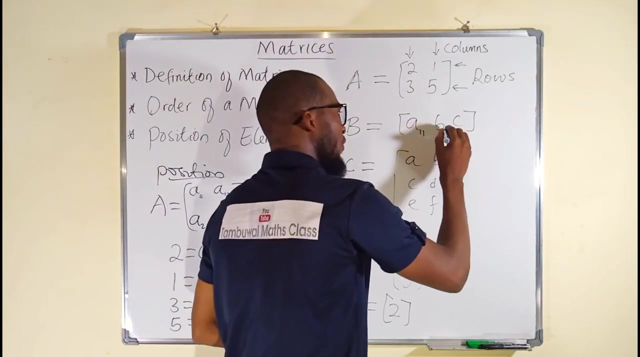 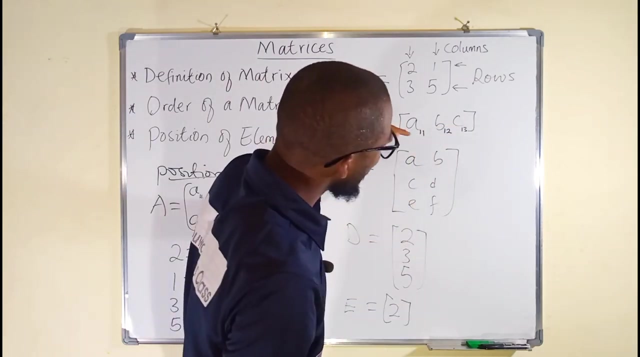 a11, a12, a21 and a22. so what about this? this one is at first row and then first column, first row. first column, first row. second column, first row, third column. you have to write them in subscript form just beneath the element. this is how to identify them. 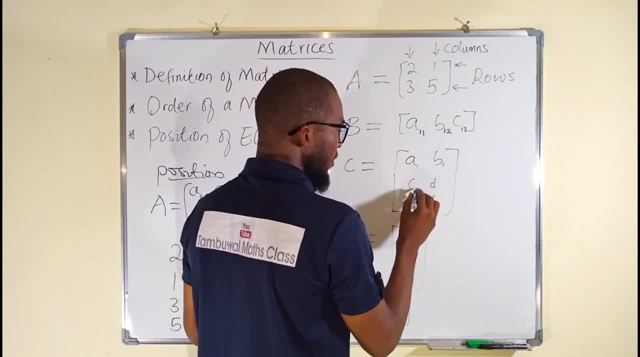 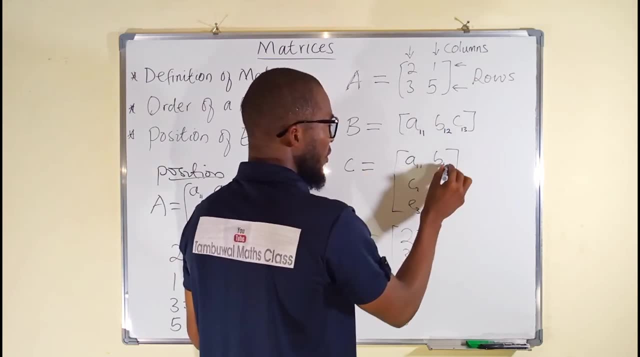 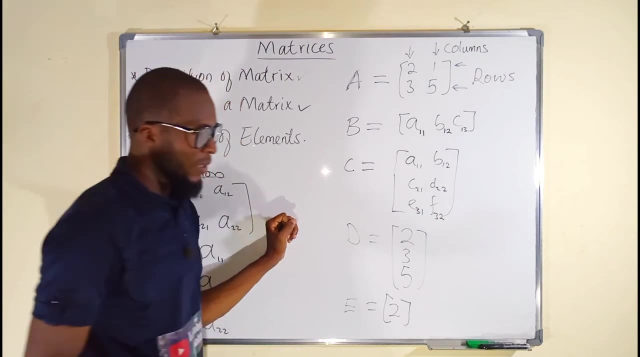 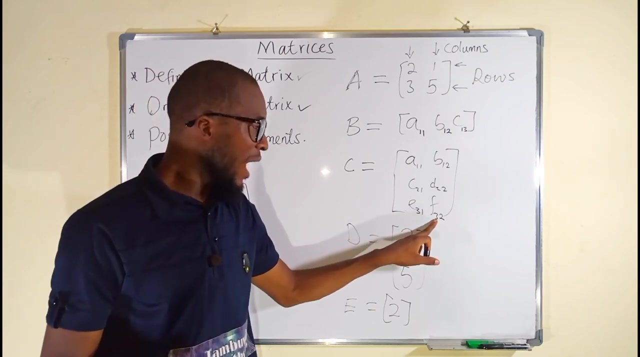 uh, this is the first row. so this is first, first, second, second, third, third. then according to column, this is first column, second column, first column, second column: first column, second column. so f is an element at the third row, second column, this one as well. you can see all. 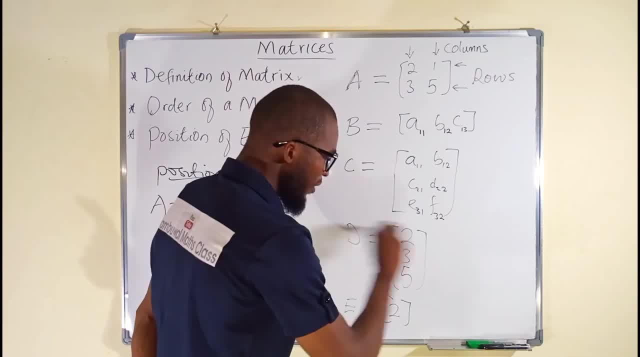 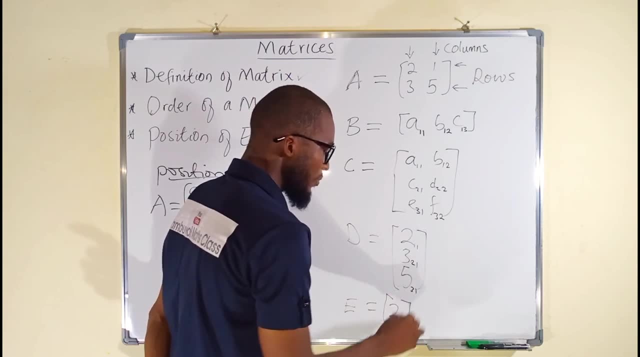 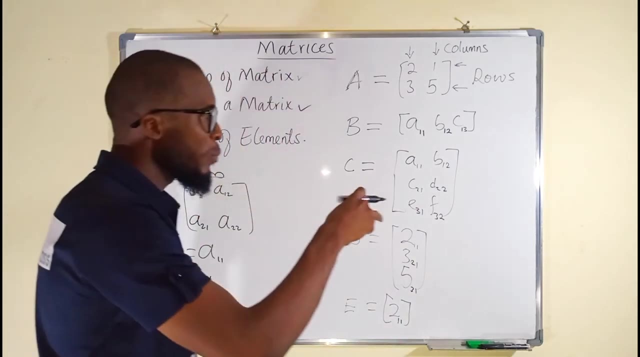 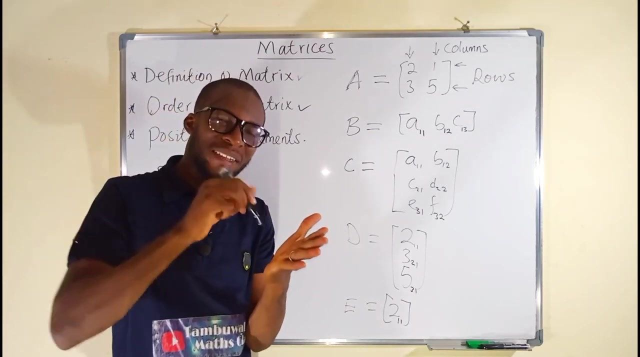 of them are from the the same column, but different rows- row 1, row 2, row 3- but all the columns are the same. what about this? first column, first row? so this is all about position. the position is said to be exactly where that element is located.